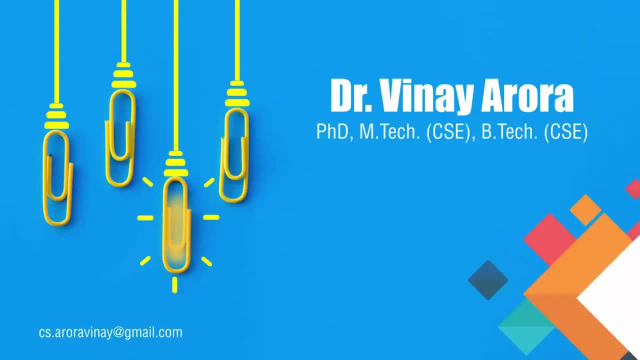 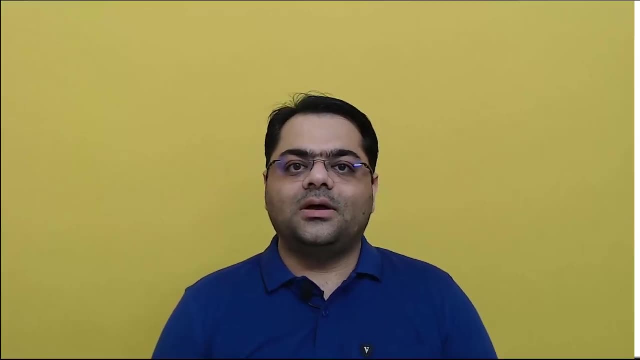 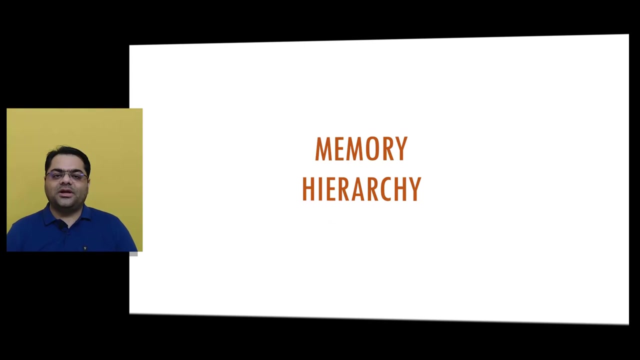 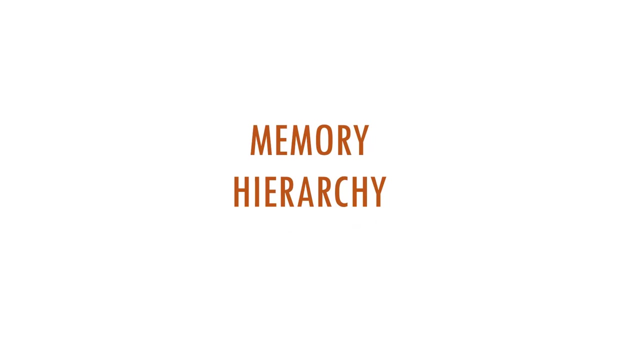 In this video I am going to discuss about memory and its hierarchy. Memory is a hardware unit that is used to store data and instruction, or you may say a computer program. Memory can be categorized as volatile and non-volatile, where volatile loses its contents in case the hardware device loses. 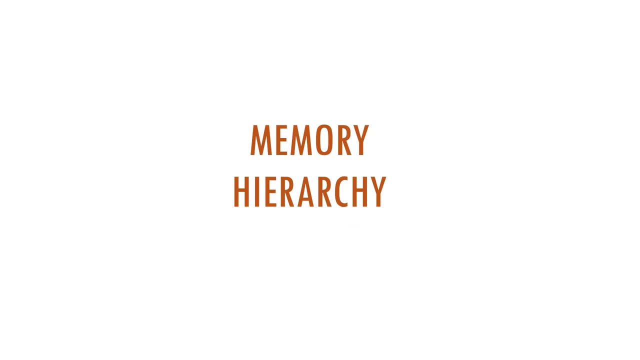 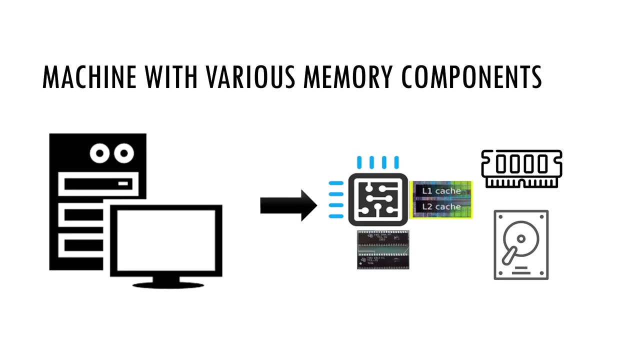 power and non-volatile, keeps its content even if the power gets off. There exist various memory units, like registers, L1-L2, cache, RAM, hard disk or you may say, SSD. These all memory units are having their own characteristics with respect to storage capacity, access speed and the cost. 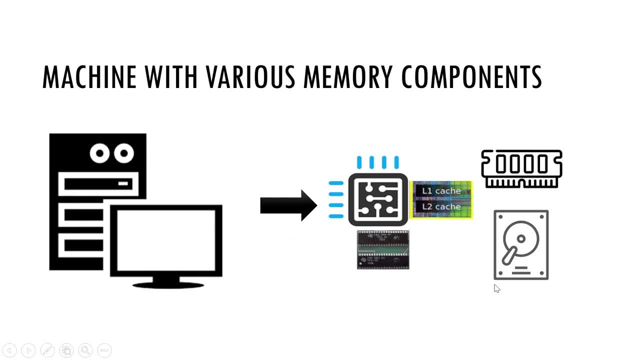 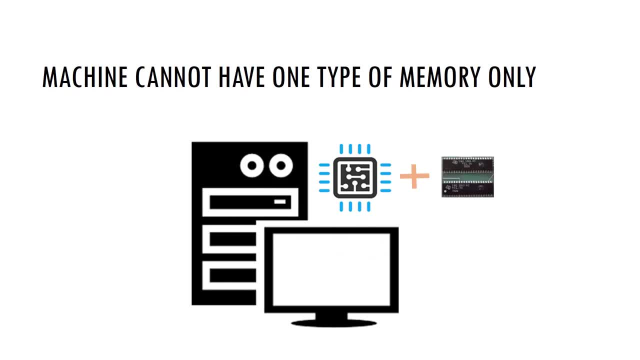 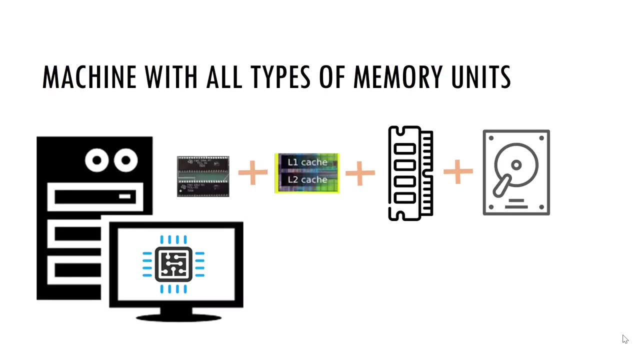 To build a computer system, we need all these memory units. We cannot have a machine with one type of memory hardware, that is, processor with either 5 or 10 gigabytes of register or cache, or the processor having 1 or 2 terabytes of RAM or hard disk only. The prime concern is performance versus cost. 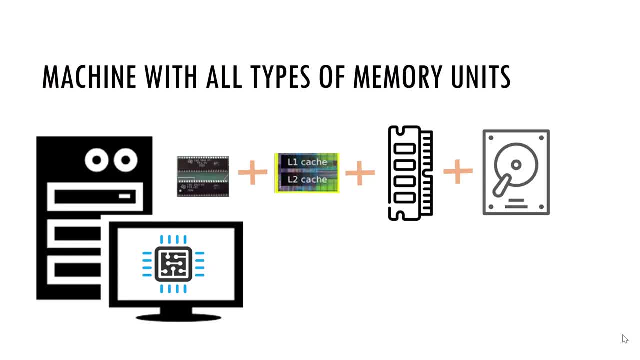 Due to the specific electronic circuitry, the cache, or registers are fast but too costly, whereas hard disk is super slow and cheap. Hence, to maintain a proper balance for cost and speed, one can think of building a system which is high in performance and affordable with respect to cost. For this we take all. 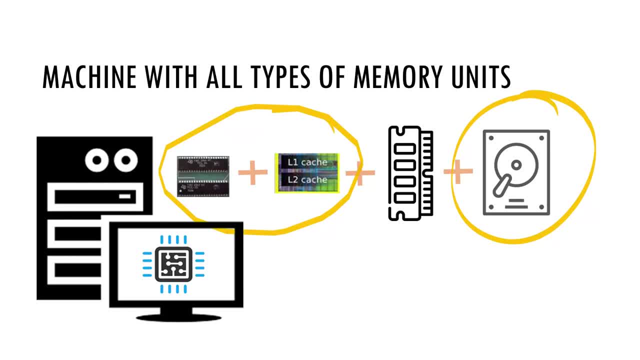 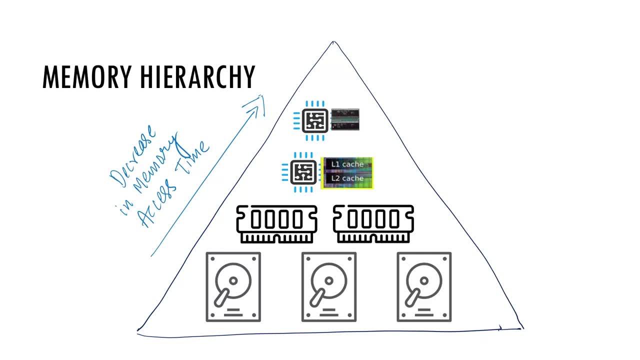 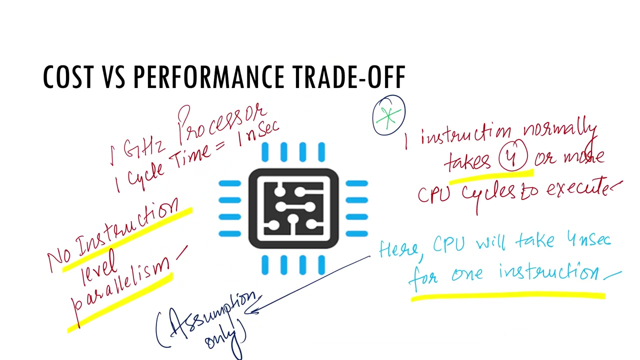 type of memory units to build a computer system. In computer system architecture, memory hierarchy corresponds to the organization of various memory units and its depiction on a pyramid-shaped structure such that the memory excess time is minimal when traversed from bottom to top. To understand the tradeoff between Performance and Cost, let us consider a scenario. Although 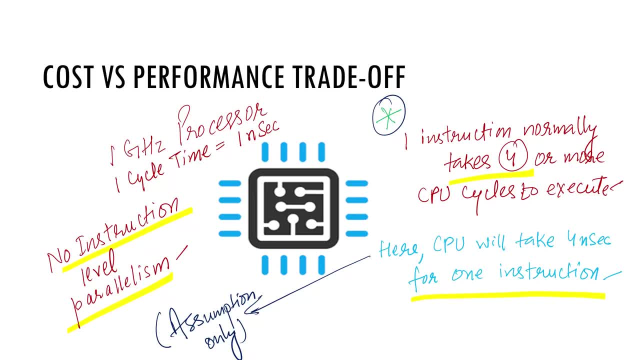 is very much dependent on the CPU type, ie its make and model. An example has been considered here, taking 1 GHz processor with a cycle time of 1 ns. Also, considering no instruction level parallelism, a simple instruction normally takes 4 or more CPU cycles to execute. Hence 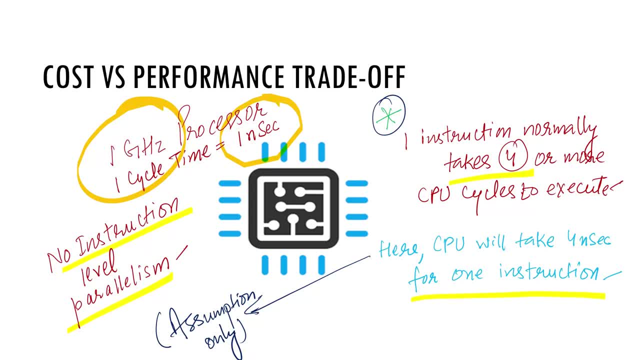 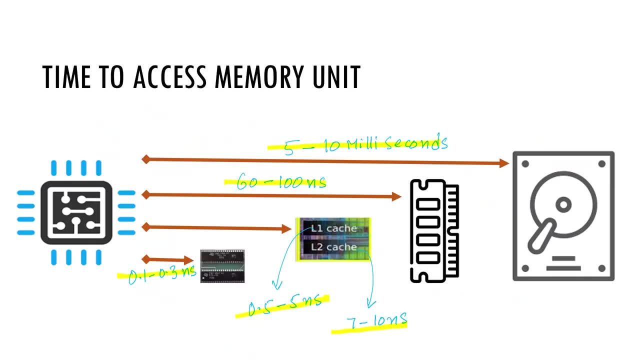 for the scenario here, we can say that the CPU will take 4 ns for one instruction. When a processor makes a request for accessing the required data from the registers, the memory access time varies between 0.1 to 0.3 ns. For L1 cache it is 0.5 to 5 ns. 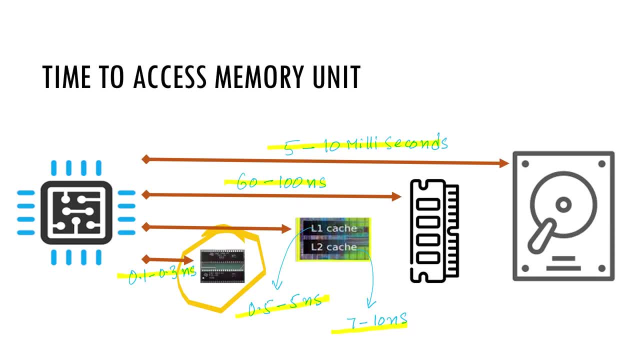 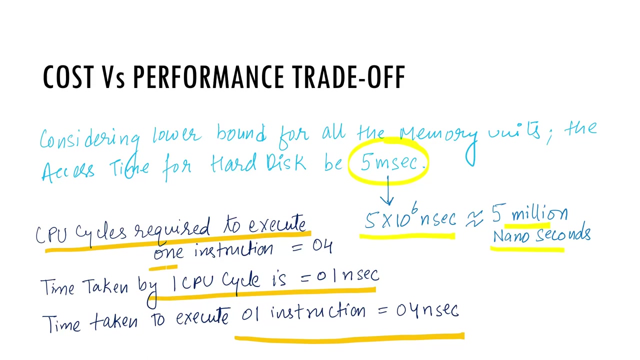 For L2, it is 7 to 10 ns, For RAM it is 60 to 100 ns and for the hard disk it varies between 5 to 10 ms. Taking the lower bound for all the memory units, the access time for hard disk storage be 5ms, and converting it to ns, it will result into: 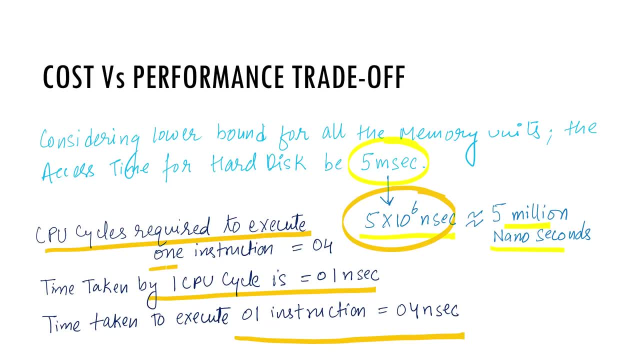 to 5 into 10, raise to power 6 nanoseconds, that is 5 million nanoseconds, And this is to access just one instruction from the hard disk. In our example scenario here, CPU cycles required to execute one instruction are 4, the time 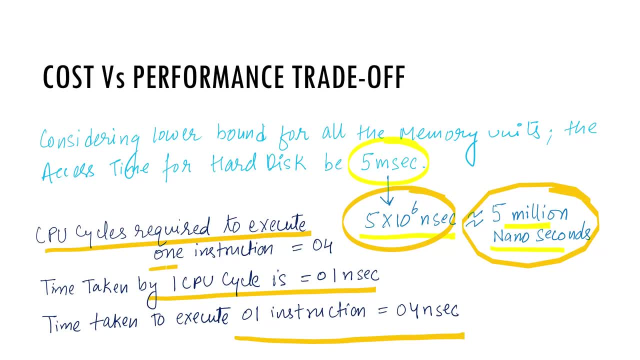 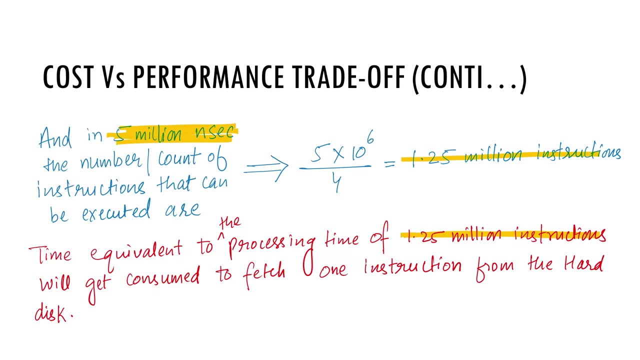 taken by one CPU cycle is 1 nanosecond. therefore we can say that time taken to execute one instruction be 4 nanoseconds. Here the number or the count of instructions that can be executed in 5 million nanoseconds are 5 into 10. raise to power 6 divided by 4, that is 1.25 million. 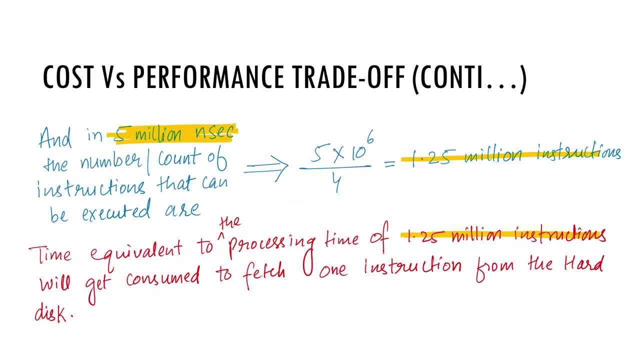 The time equivalent To the processing time of 1.25 million instructions will get consumed here to fetch one instruction from the hard disk, And hence the CPU has to sit idle for this much time as a wait, because the processor will process an instruction using 4 CPU cycles and look for another instruction to process. 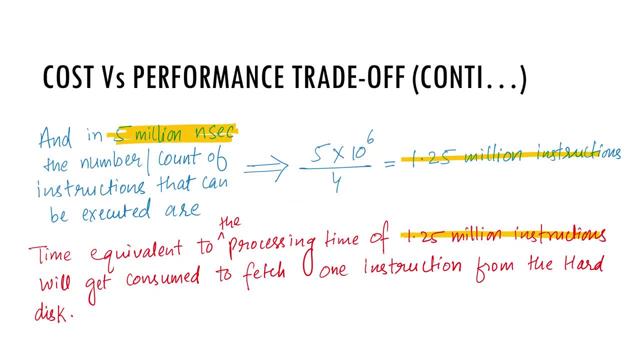 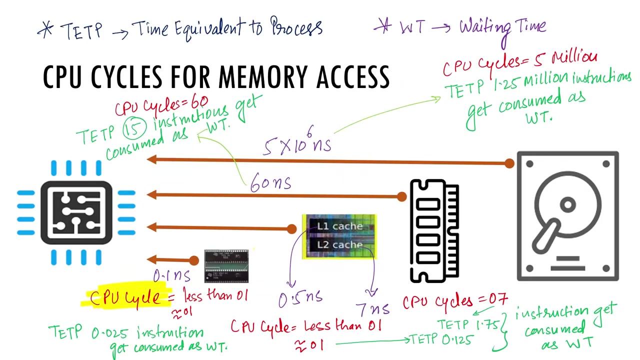 But here CPU needs to wait For next instruction to come, as it's fetching will take the time equivalent to the processing time of 1.25 million instructions. This idle, or you may say useless, sitting will degrade the performance of the CPU. The comparison among the memory units can be visualized on the basis of CPU cycles. 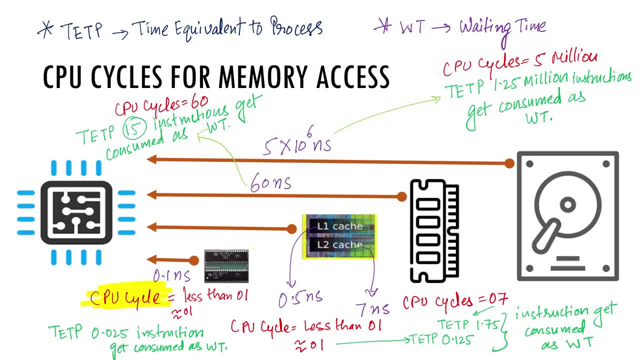 which get consumed By the processor processor for accessing the data. This be 1 for the register, 1 to 7 for cache, 60 for RAM and 5 million for the hard disk, considering 1 nanosecond for one CPU cycle. 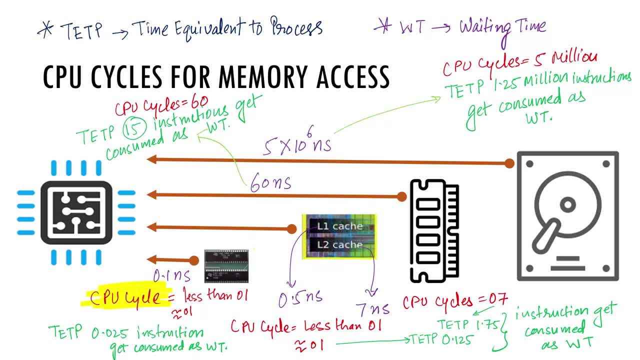 The memory units, like hard disk RAM cache register, can also be compared on the basis of count of instructions that could be processed in the wait time for which the processor sits idle. So in case of data access from the registers, the access speed is very fast and processor 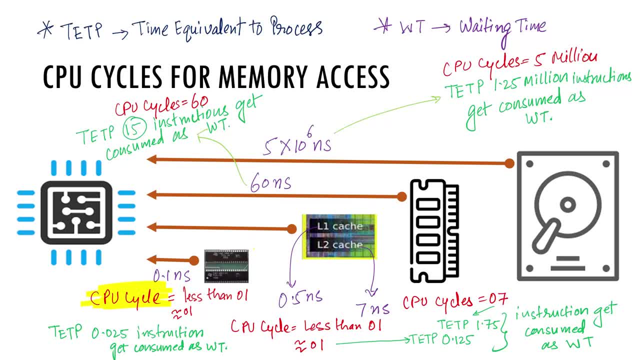 will wait just for the time equivalent to processing 0.025 instructions. For L1 and L2 cache, time consumed is equivalent to processing 0.125 and 1.75 instructions respectively. For RAM time equivalent to process 15 instructions will get consumed as waiting time. 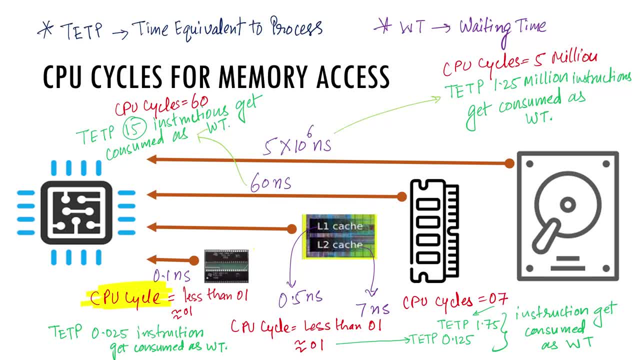 And for the hard disk the time equivalent to process 1.25 million instructions will get consumed Here. data access from either registers cache or RAM is comparatively faster as compared to the data access from hard disk, But cost factor will make it infeasible to build a machine having either register cache.